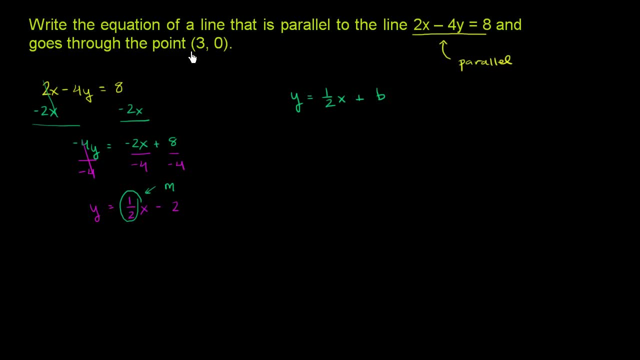 So now we need to figure out how to figure out b, And to do that we have this information right over here On this line, the one we care about. when x is 3, y is 0.. When x is 3, y is equal to 0. 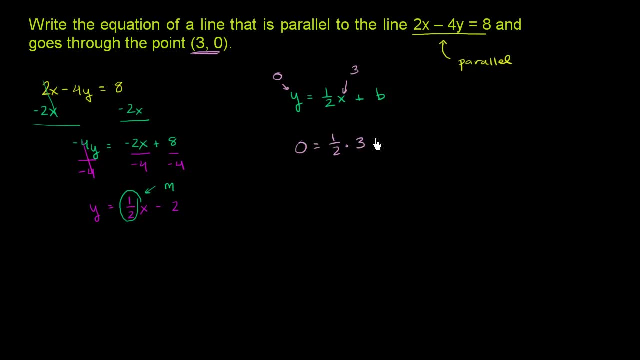 Or we could say: 0 is equal to one-half times 3 plus b. We just have to find a b that sets up this equation. so then, when x is equal to 3, y is equal to 0. So we get: 0 is equal to 3 halves plus b. 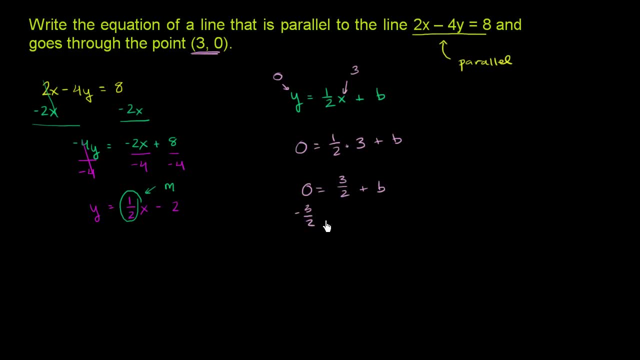 Subtract 3 halves from both sides And we get negative 3 halves is equal to b Or b is equal to negative 3 halves. So we have the equation for our line. That is now parallel to this equation and goes to the point. 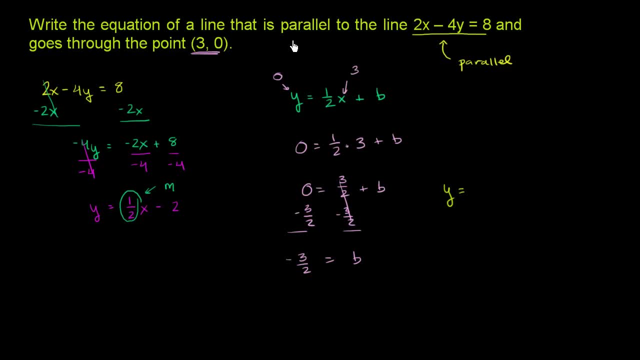 It is, y, is equal to it, has the same slope as this guy up here. one-half x, And now we know it's y, intercept Minus 3 halves And we are done. And actually, if you're interested, you could graph these two and see that they're parallel. 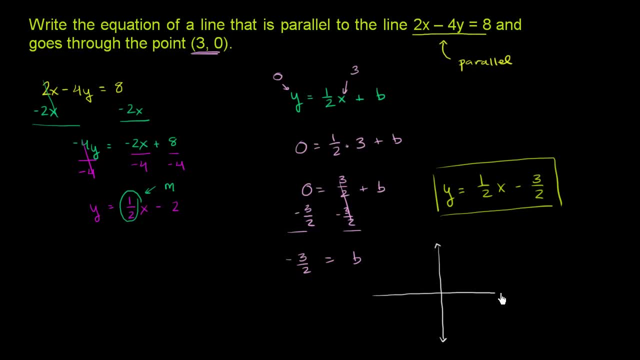 So if you were to graph these, I'll do just a very rough graph really fast. So this is my y axis, This is my x axis, This line up here- I'll do it in blue: This line up here, which is the same thing as this line right over here. 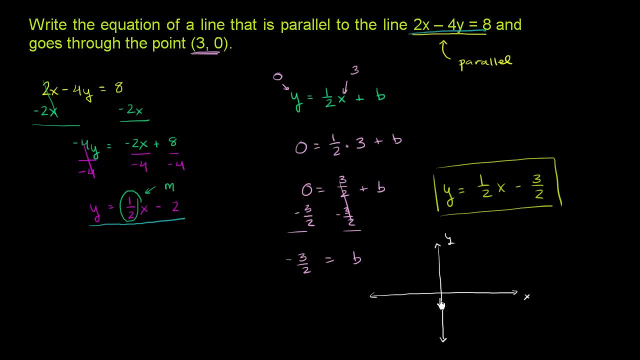 I just algebraically manipulated it. It has a y intercept at negative 2.. So negative 2.. So 1, 2 at negative 2. And it has a slope of one-half. So that means that for every 1 it goes over, it only goes a half up. 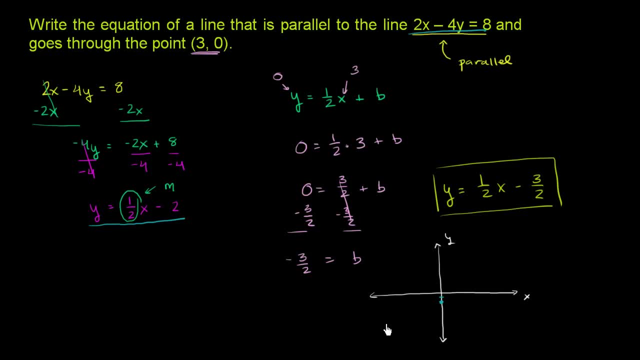 Or for every 2 it goes over, it only goes one up. So it's going to look something like this. I'll try my best To draw it. It's going to look something like that. And so this line over here, its y intercept is at negative 3 halves. 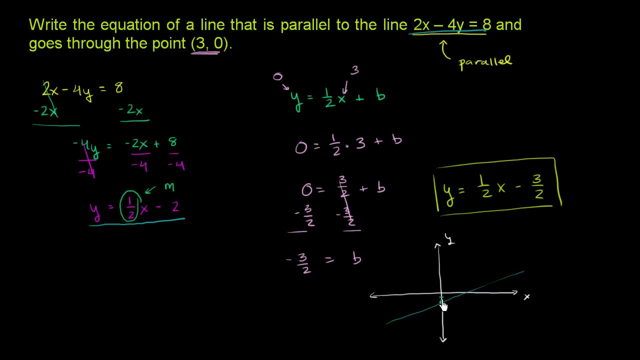 And negative 3 halves is the same thing as negative 1 and a half, So it's going to be right over here, It's going to be right above it, Right over there, And it has the exact same slope, So it's going to be right above it.